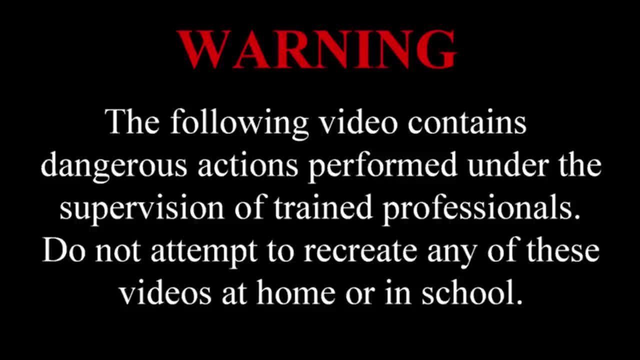 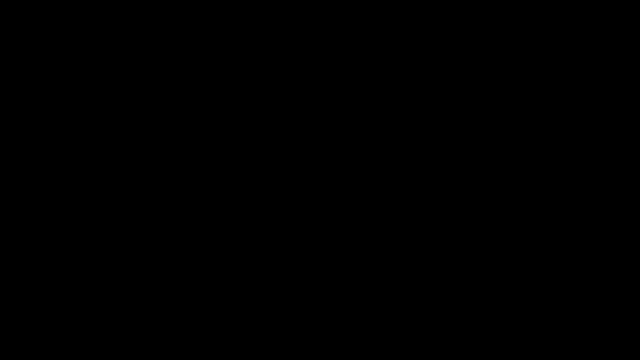 Warning: The following video contains dangerous actions performed under the supervision of trained professionals. Do not attempt to recreate any of these videos at home or in school Viewer discretion advised. Hello, I'm Mr Bazanson, science teacher at Oroville High School. 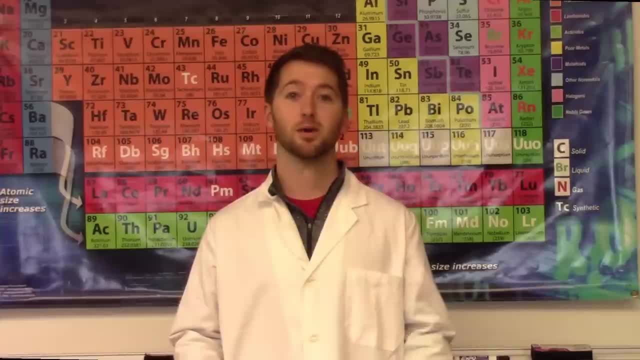 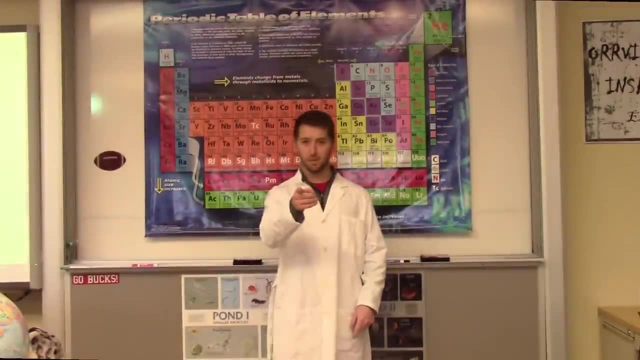 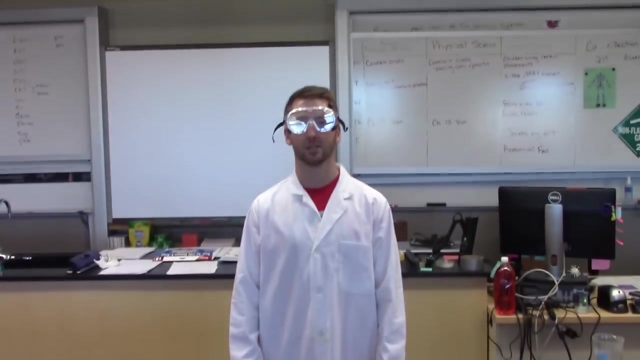 Today, we're going to talk about one of the most important things in a science classroom, and that's lab safety. Specifically, we're going to talk about the do's and the don'ts of lab safety. Do not ever wear open-toed shoes, such as sandals or flip-flops, on lab days. 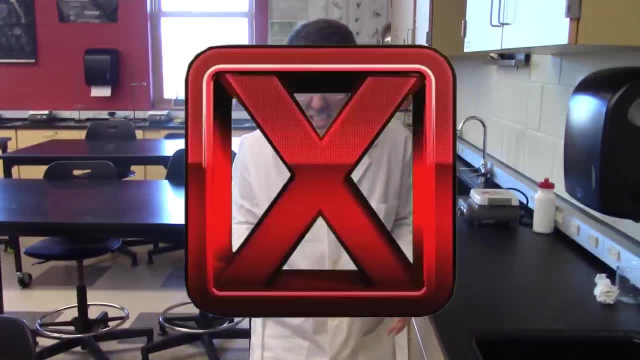 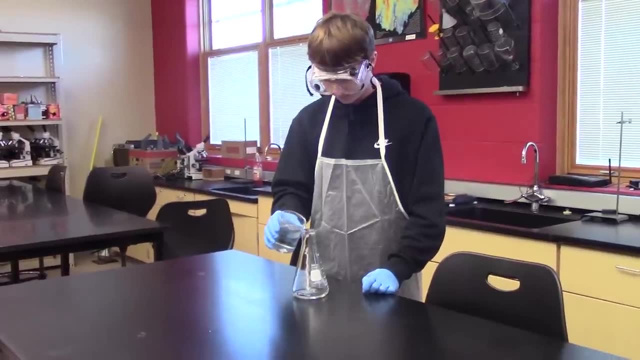 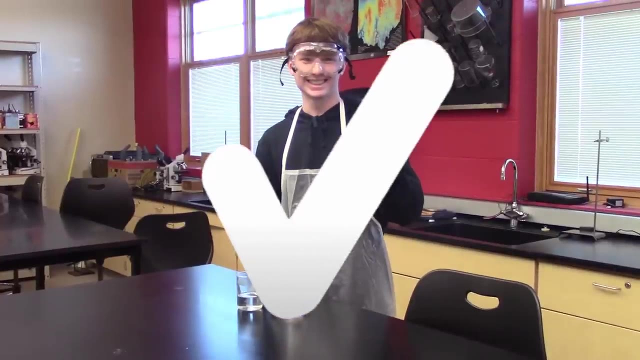 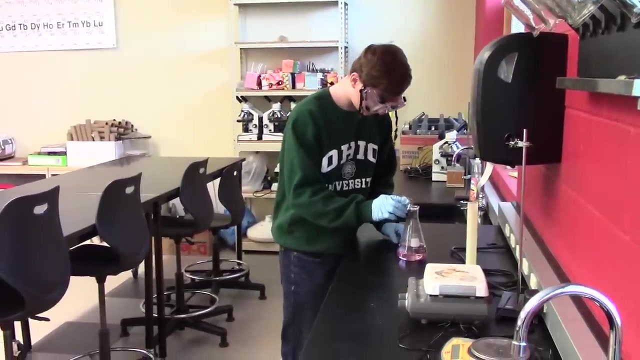 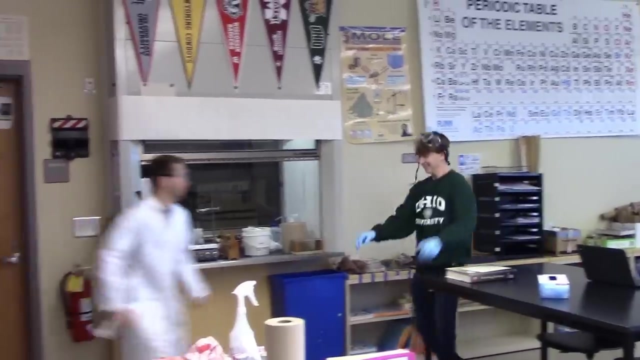 Ouch, Ouch. Do Always Make Make sure to wear your personal protective equipment. Do not ever touch your face or eyes after handling chemicals. Cole Eyewash station right here. Hurry up, Hurry up. 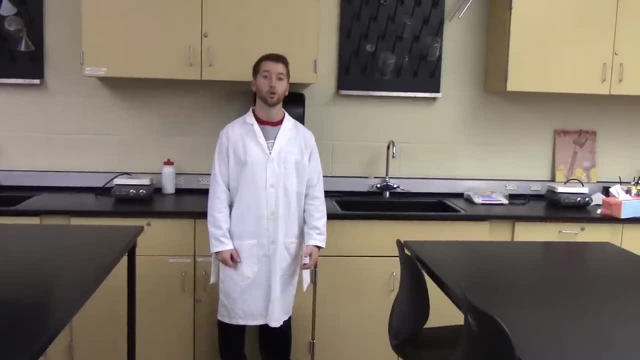 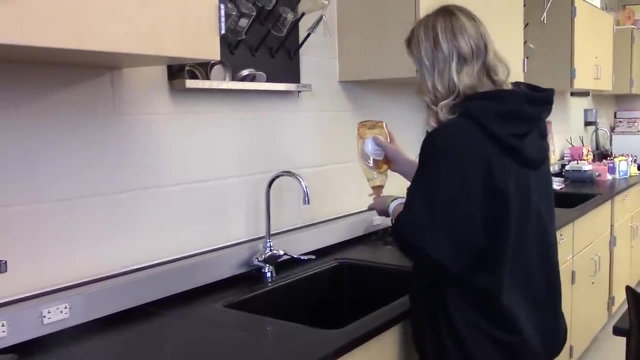 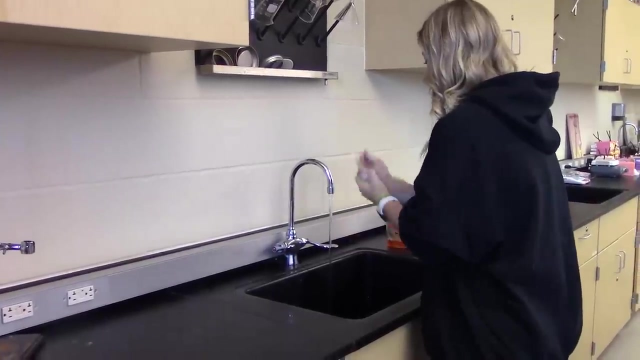 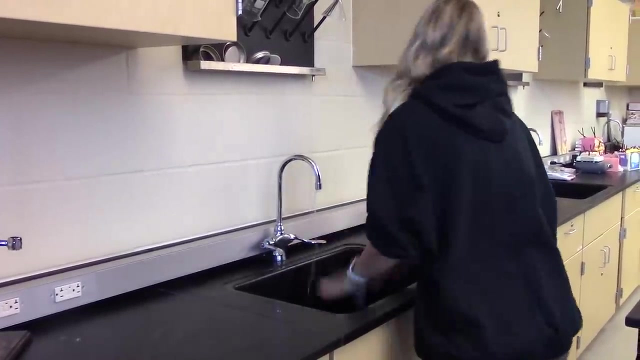 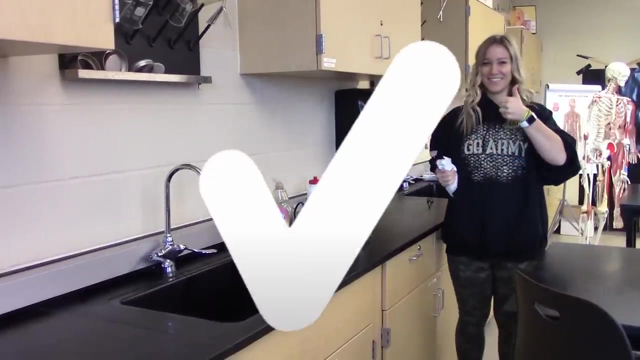 Do Always Make sure to wash your hands before and after a lab. Do Always Make sure to wash your hands before and after a lab. Do Always Make sure to wear your little shoes wearing a mask. Do not ever eat or drink during a lab experiment. 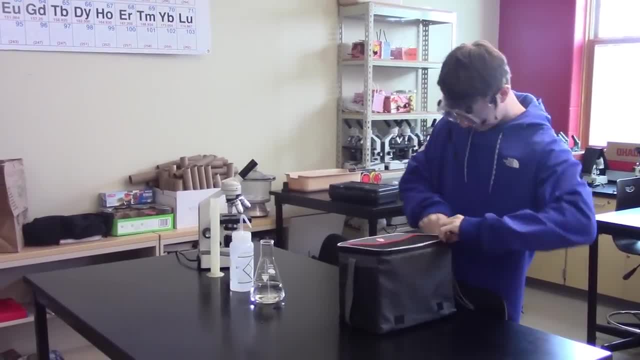 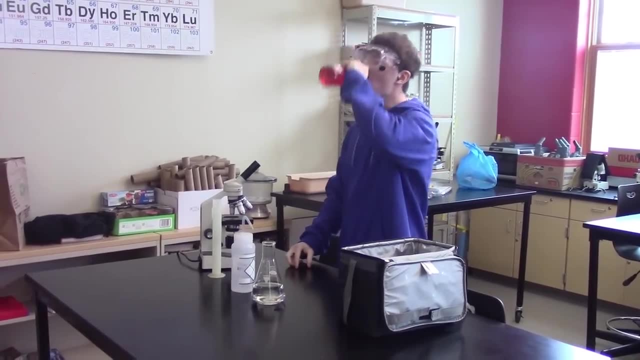 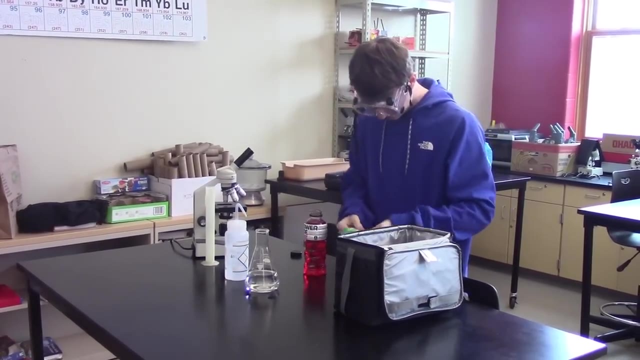 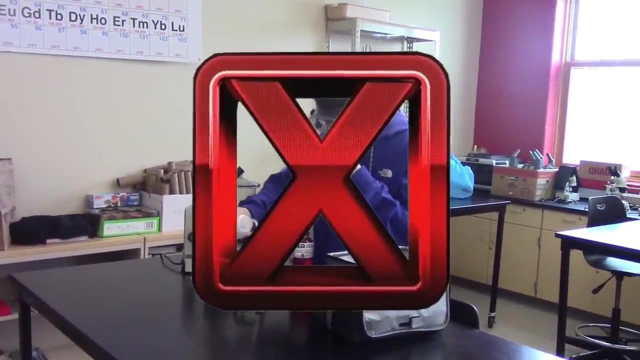 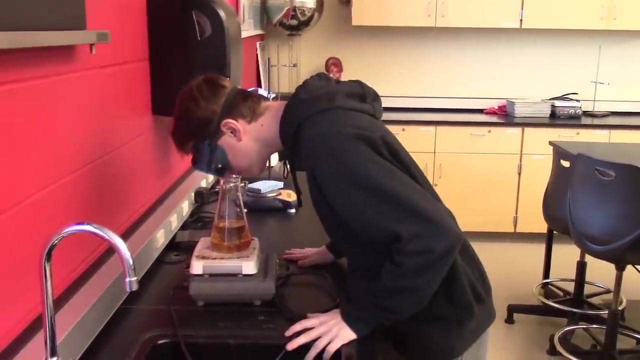 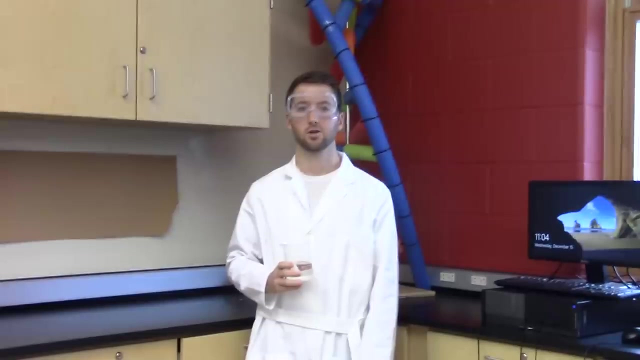 Do not ever eat or drink during a lab experiment. Do not ever eat or drink during a lab experiment. You're like aving compete right. Ah, PB&J, Love you mom. Do not ever smell or inhale an unknown chemical. 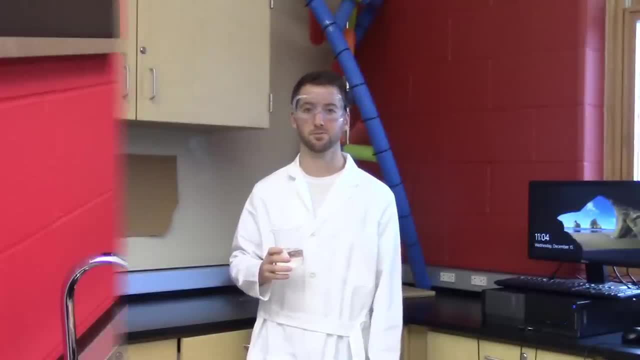 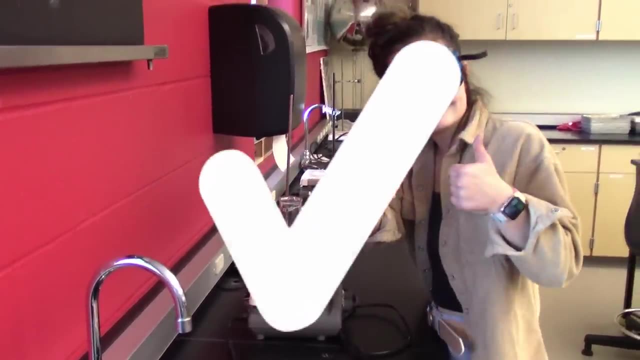 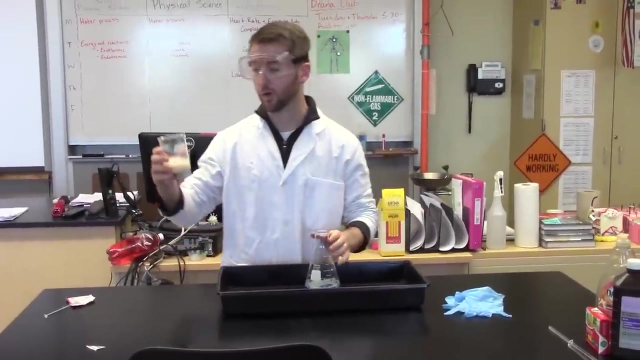 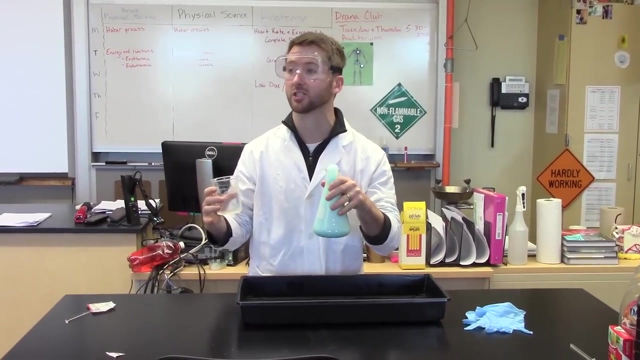 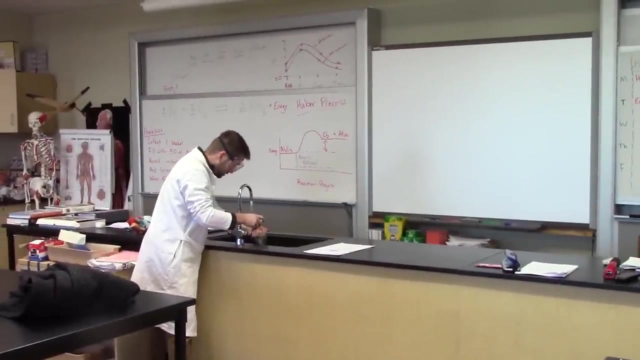 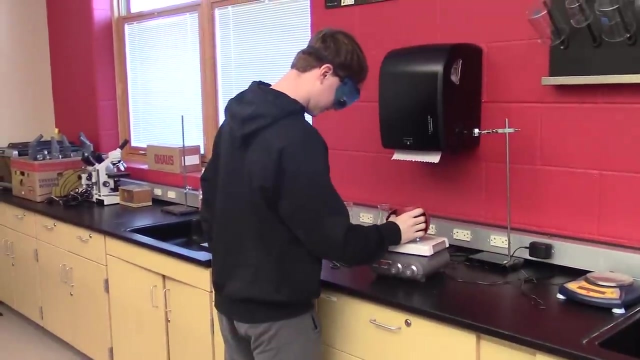 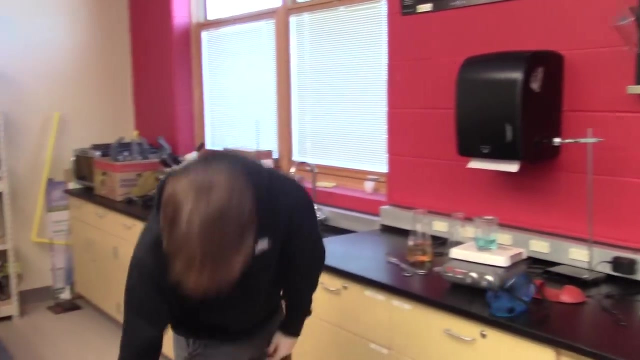 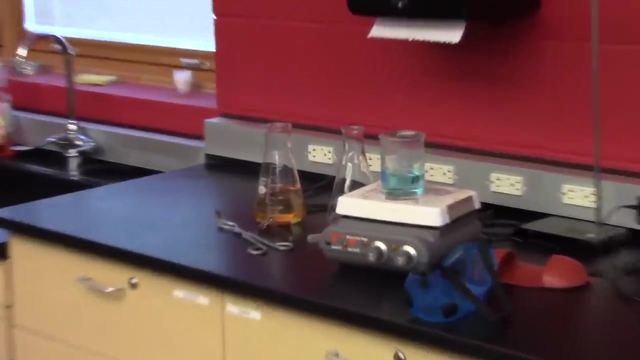 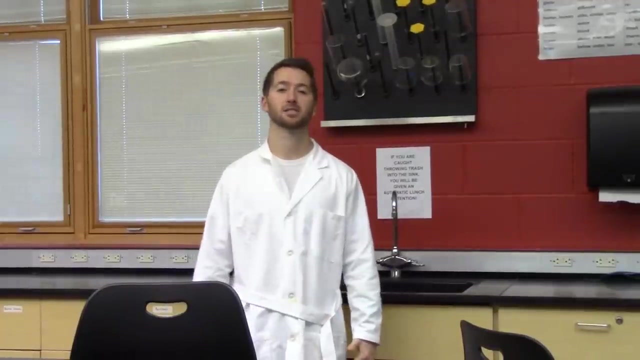 Do use the wafting method if you must smell a chemical. Do not forget to wear gloves when handling strong acids or bases. Do not leave your lab area without first cleaning up. Do not ever mix chemicals unless instructed to do so specifically in your lab directions. 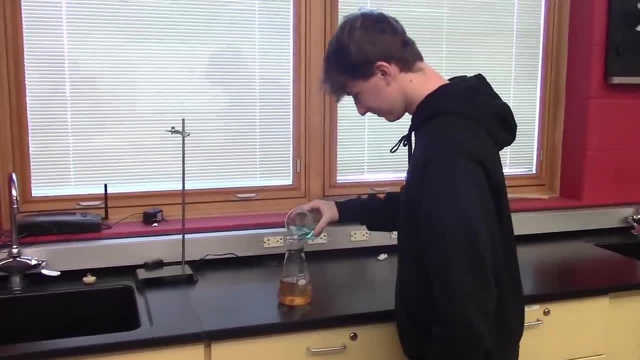 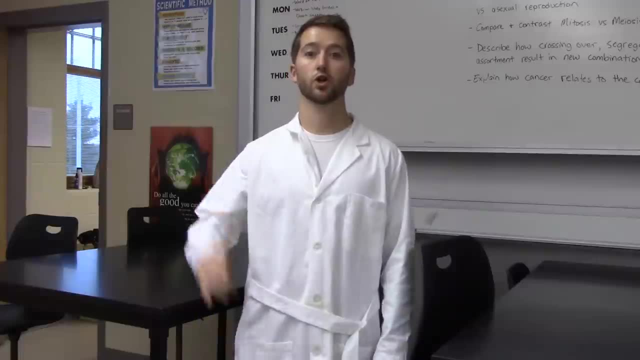 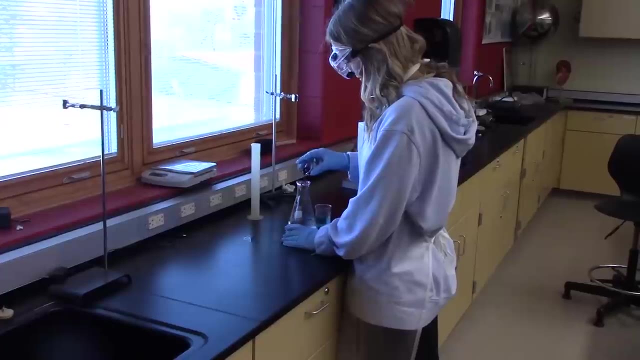 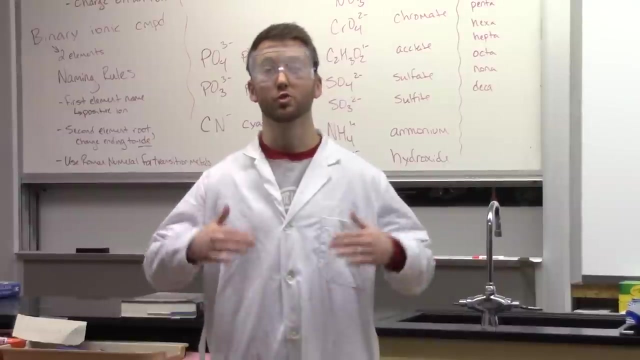 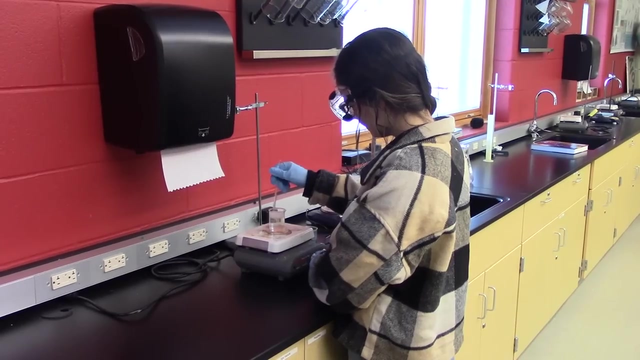 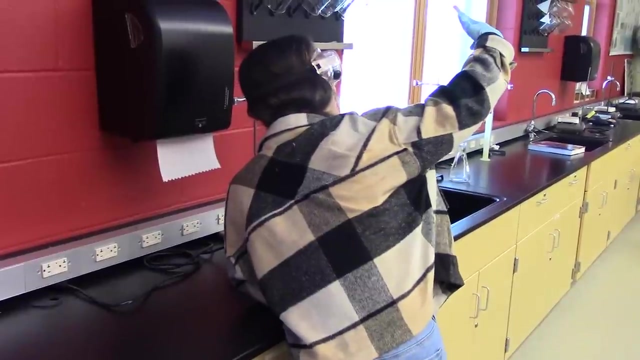 Oh yeah, this should work. Do always report any spills or accidents to your lab instructor. Mr B, I spilled the chemicals. Do not use your cell phone during a lab. Lily, look, Whoa. Lily, Lily, Oh. 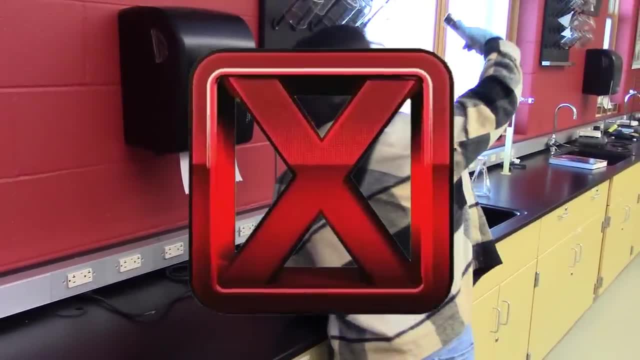 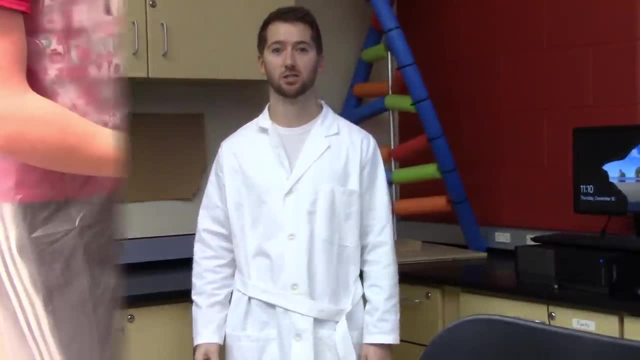 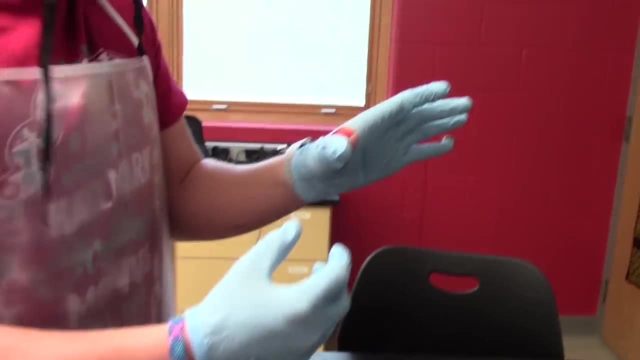 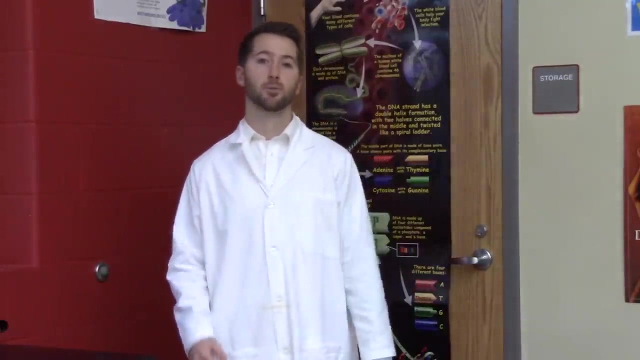 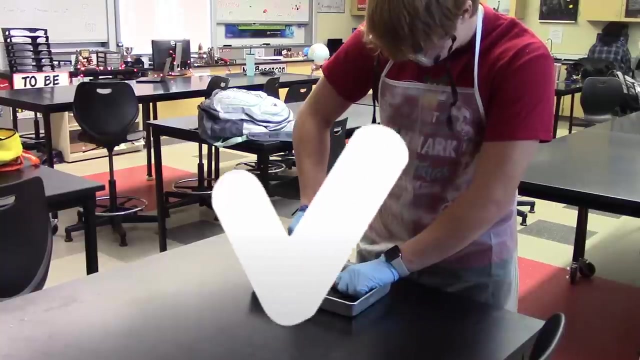 I'm in biology class. Do not ever cut towards your hand when using a scalpel during a lab dissection. Do always use caution when handling sharp objects such as knives and scalpels. Oh, that's juicing. Do not ever engage in any type of prank or 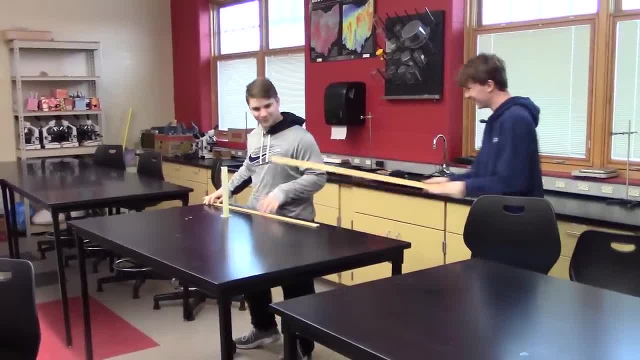 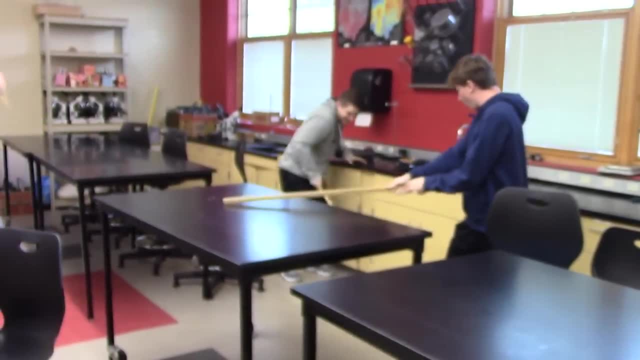 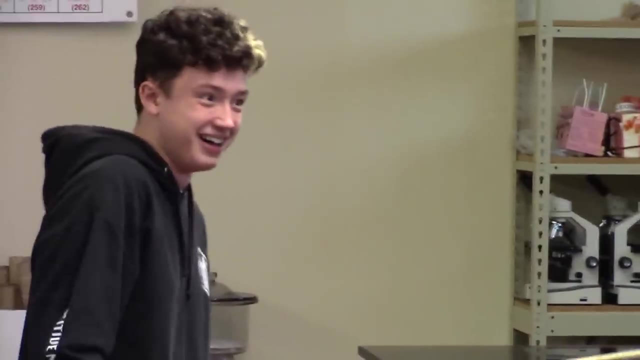 horse play during a lab activity. I want to join guys. Uh, Bzzzzzzzzz, Bzzzzzzzzzzz, Bzzzzzzzzzzz. Do not ever leave backpacks and other materials in the aisles during a lap. 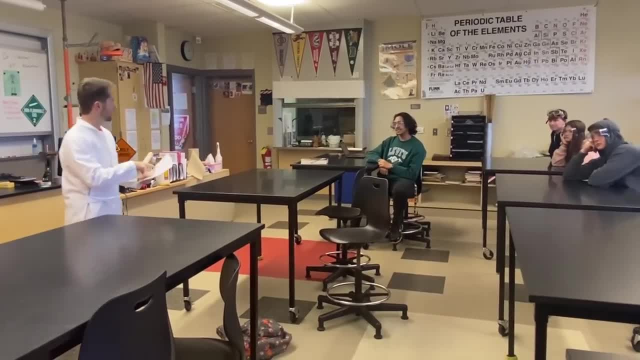 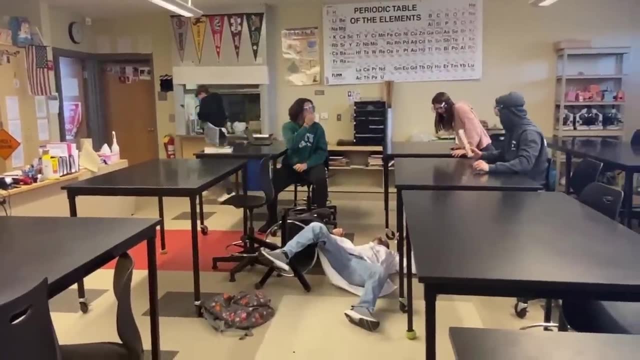 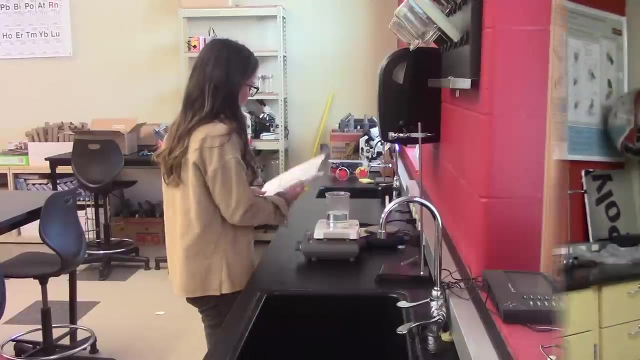 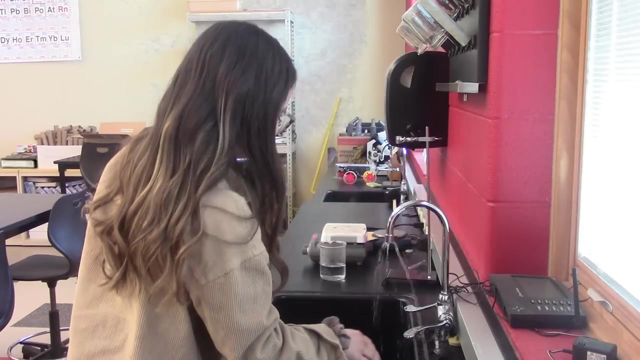 Okay, guys, just show all of your graduated cylinders and if you look here on number three in the lap, Do not ever touch hot glassware with your bare hands, Alright. so I think you have to take this: Do use tongs or rubber grabbers whenever you are handling hot glassware. 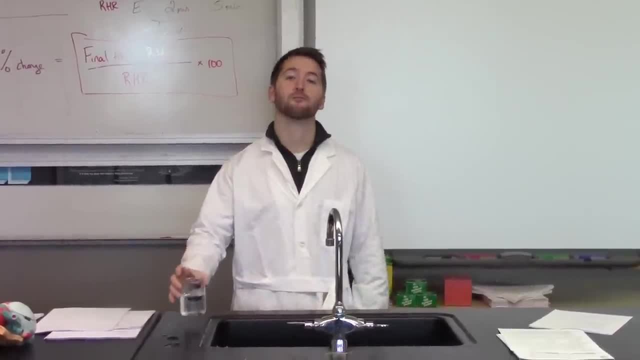 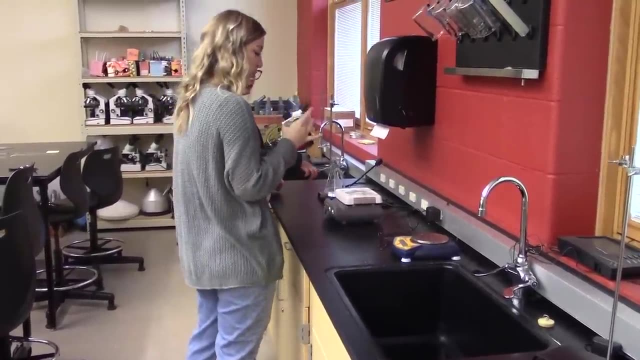 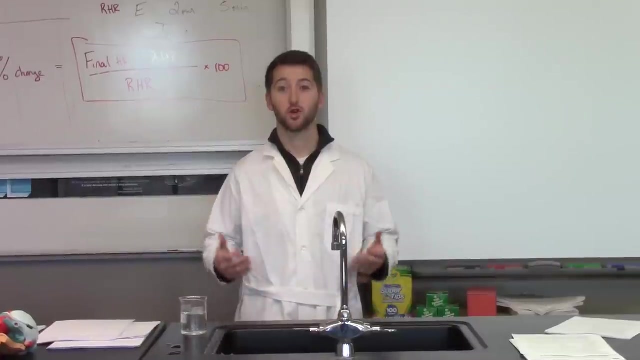 Do not ever dump a chemical down the sink without first asking your teacher for permission. What should we do with this now? I don't know. you could probably just pour it down the sink. Do always ask your teacher for permission before dumping chemicals down the sink. 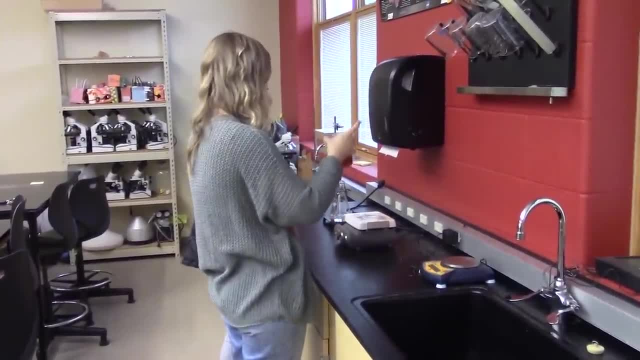 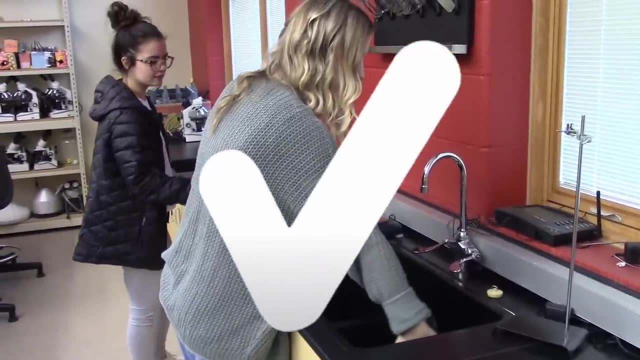 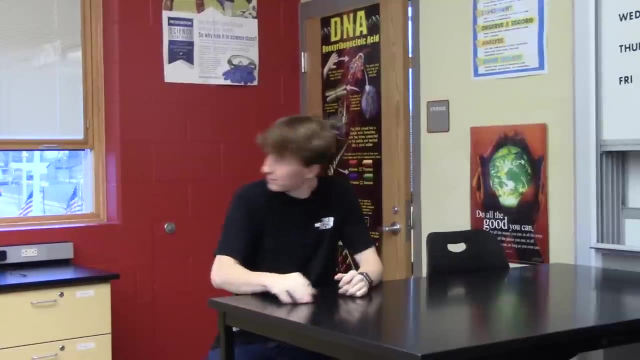 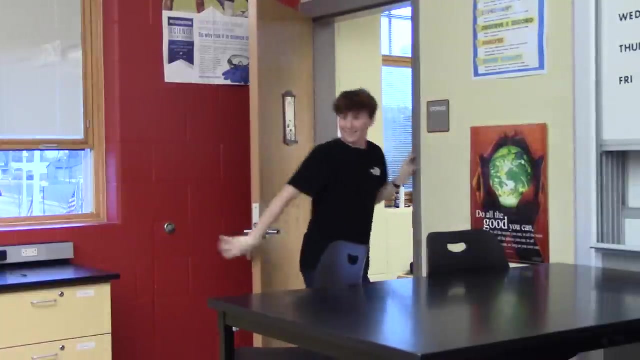 What should we do with this now? Hey, Mr B, can we just pour that down the sink? Yeah, Okay, Do not ever go into the bathroom. Do not go into the storage closet without permission from your teacher. Hey, get out of there. 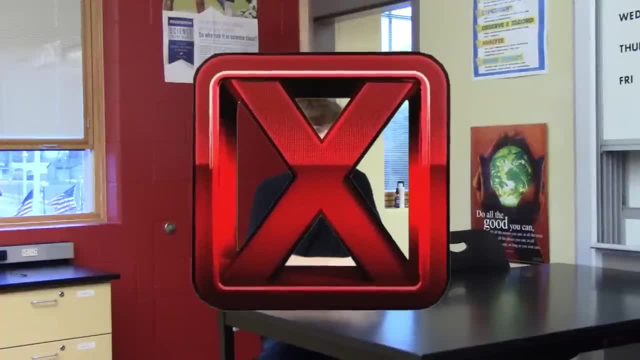 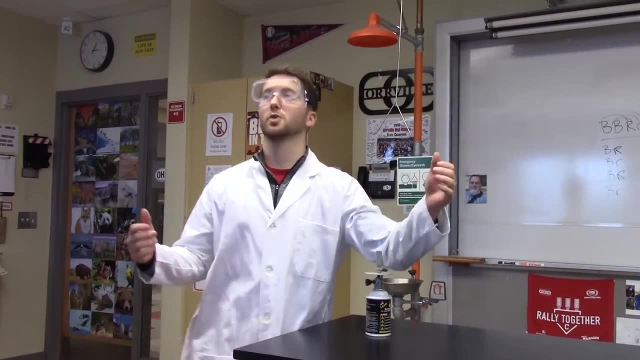 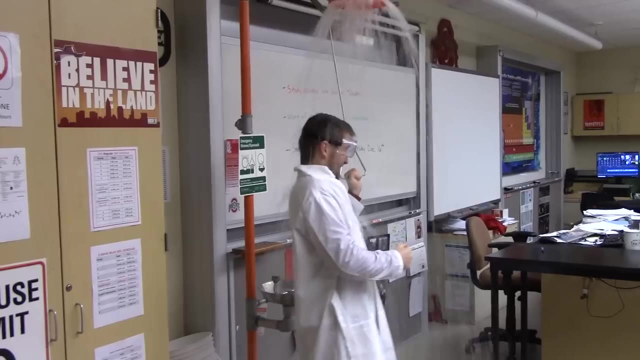 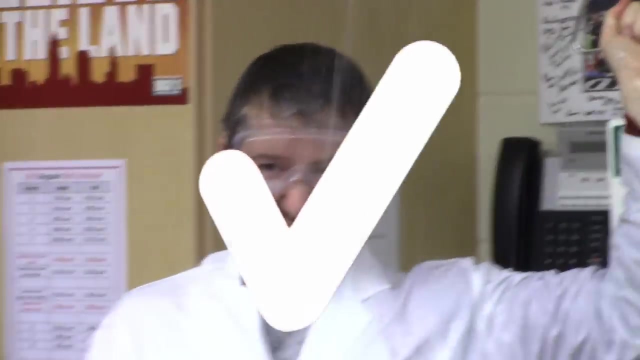 Not to detention. Do not ever leave an open flame Bunsen burner unattended. Alright class. so today, here's what we're going to do. We're going to make sure that we're always going to be. Do Always make sure you know where the shower is in a science classroom. 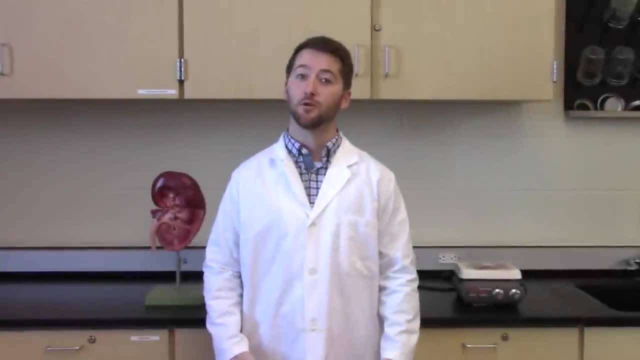 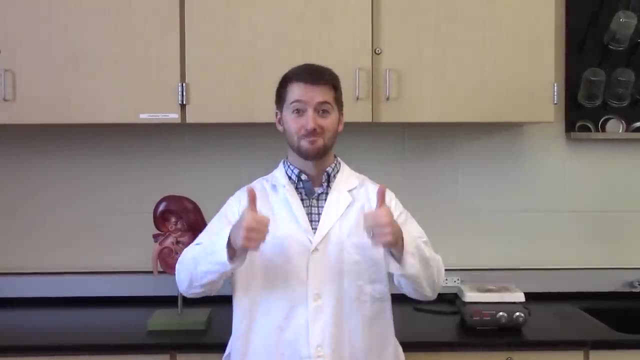 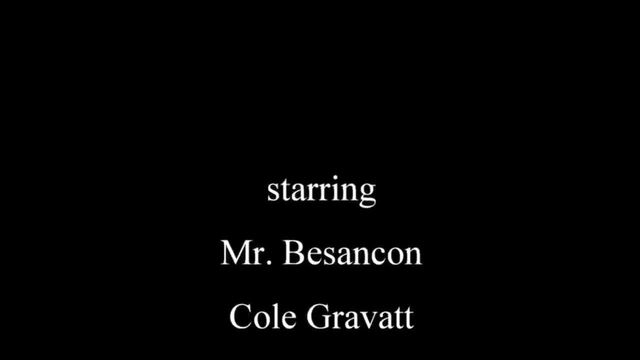 Remember kids: if you follow these simple do's and don'ts of lab safety, you will be sure to have a safe, fun year in your science classroom. Remember kids: if you follow these simple do's and don'ts of lab safety, you will be sure to have a safe, fun year in your science classroom. 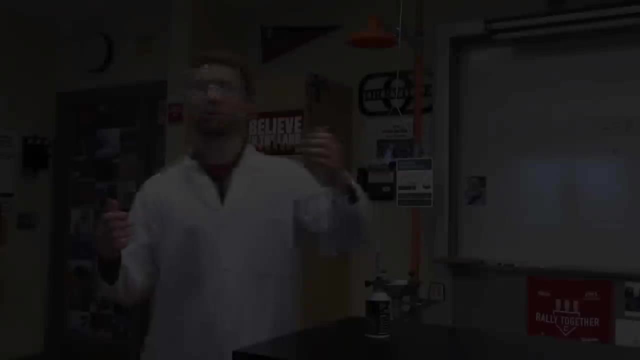 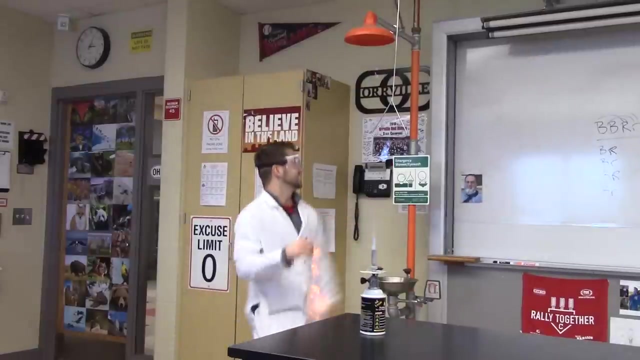 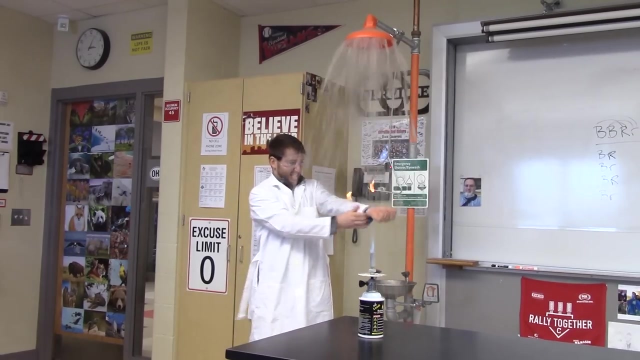 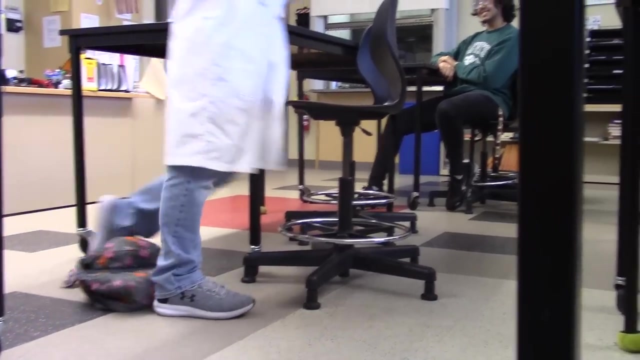 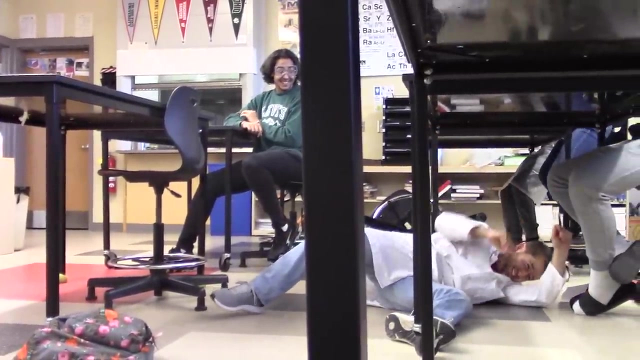 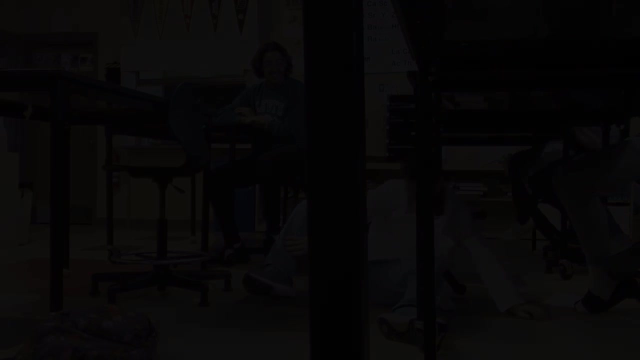 How long will you take to be in a science classroom? Well, I'm not sure I know where the shower is. I don't know. 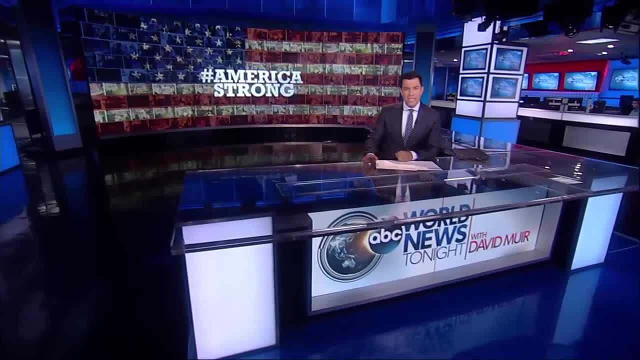 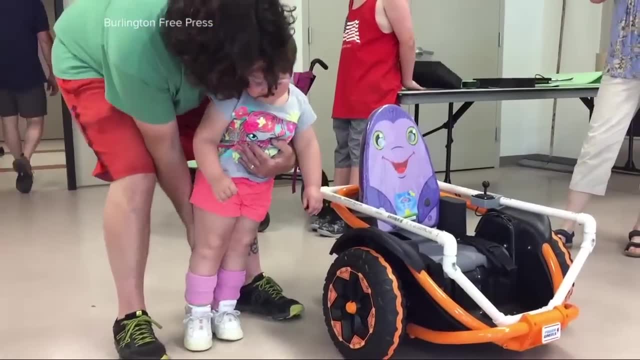 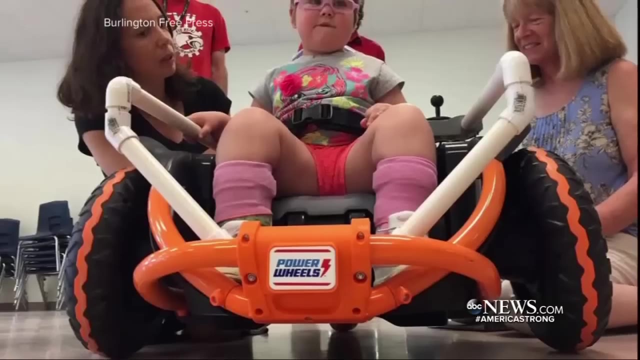 Finally, tonight, America Strong, the four-year-old girl in need of a wheelchair and the 17-year-old high school inventor turning a toy into a life-changing gift. You're about to watch as four-year-old Miley Brochu's life is about to change. Put your feet right in here. It may look. 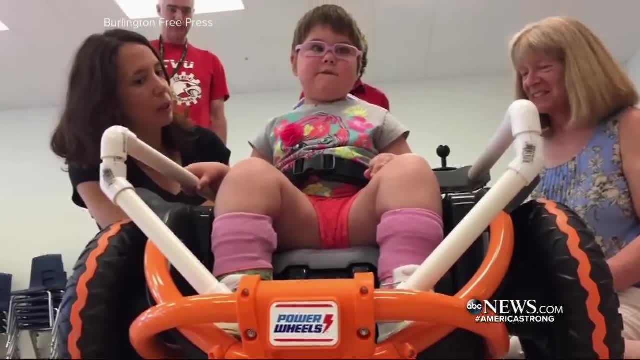 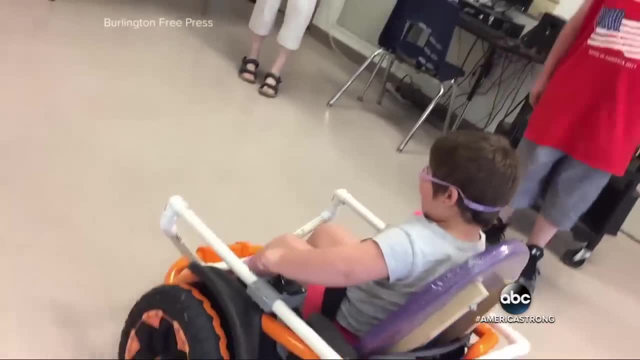 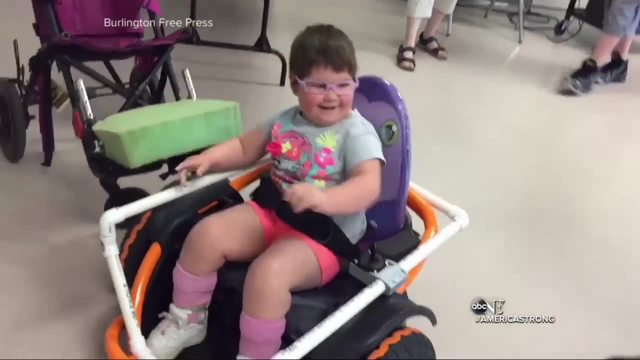 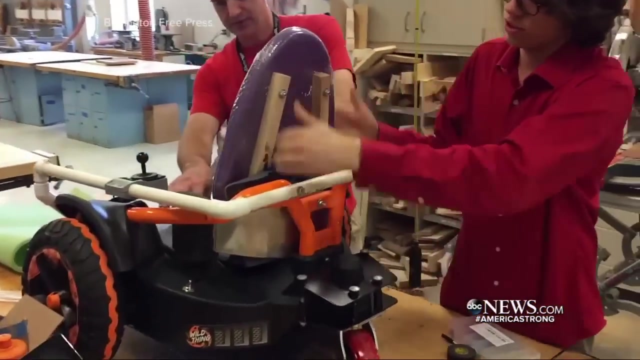 like just a toy, but this souped-up power wheel may be Miley's first chance to get around by herself. There you go, Look at you. Miley is a shaken baby survivor and she can now move around by herself because of a high school science project. Seniors at Champlain Valley Union High. 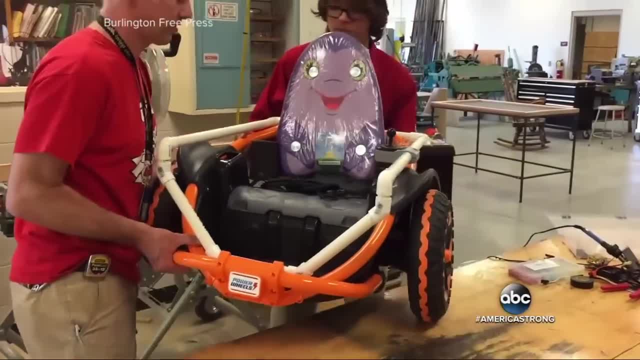 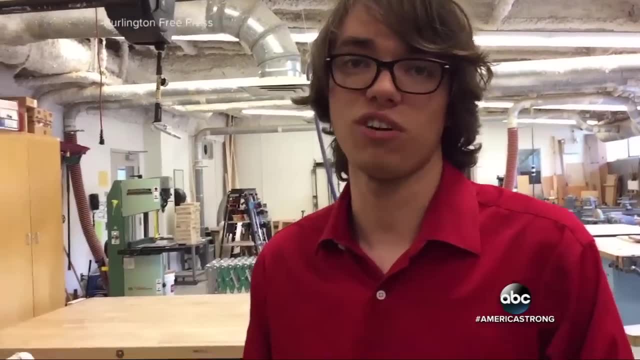 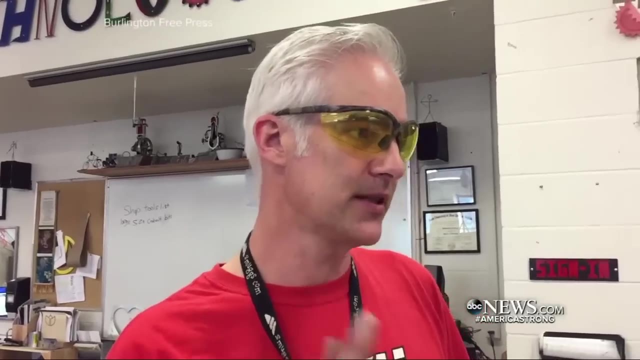 in Vermont built the mini mobility scooter in the robotics lab. It's for this girl here. She can't really walk, and so this is going to be her first opportunity to be able to move herself. Turn it a little, A little bit this way: Less speed, Do a lot of high-tech stuff here and the big piece that this. 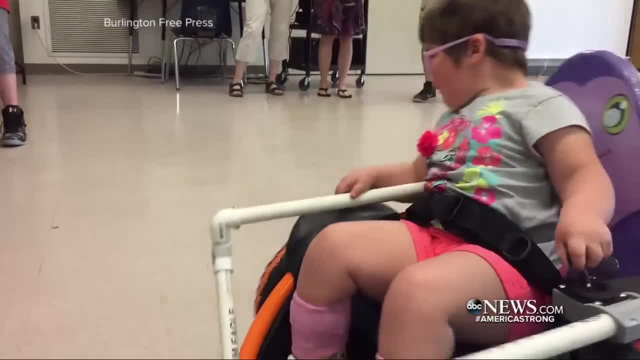 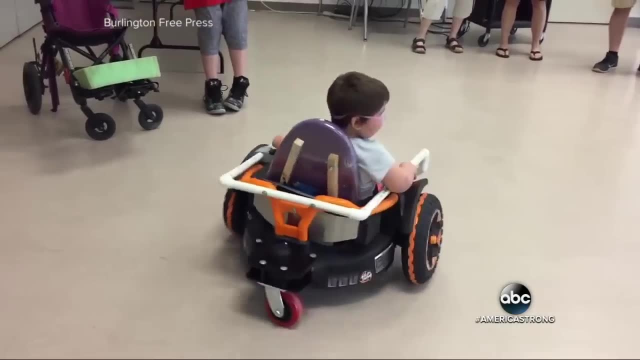 project tied in was empathy, A project that changed a life and those students seeing it up close. Miley's therapist saying: by giving the little girl the power to move, they're going to help her with more than just transportation Kids who are unable to walk. if you give them the 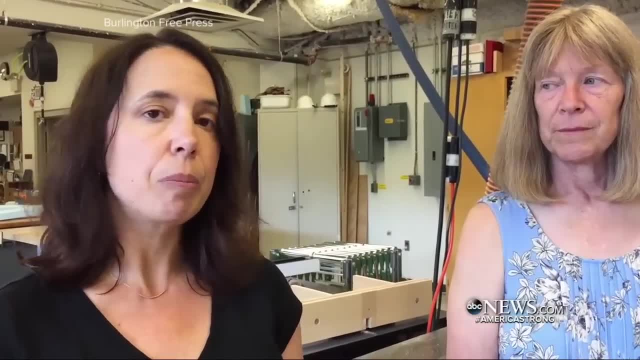 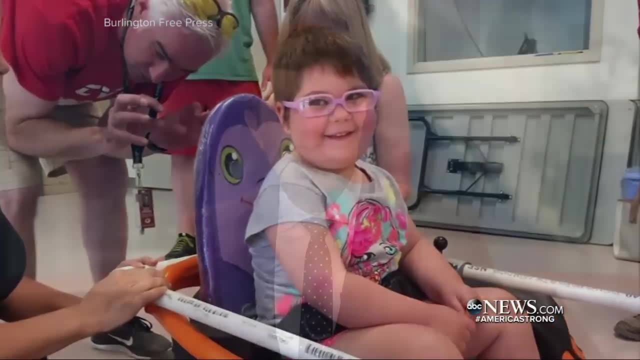 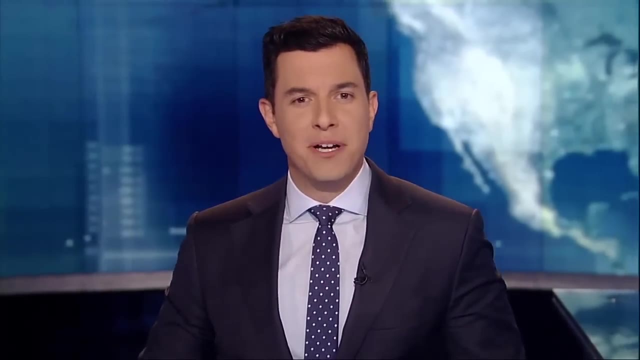 ability to independently move, then their other motor skills increase, their social skills increase. That just encompasses everything. You give them that independence. So tonight we salute teen inventor Wilhelm Hillier and Miley Brochu as well for being America strong. Thanks so much for watching on this Monday night. I'm Tom Yamas. I hope to see you right back here tomorrow.